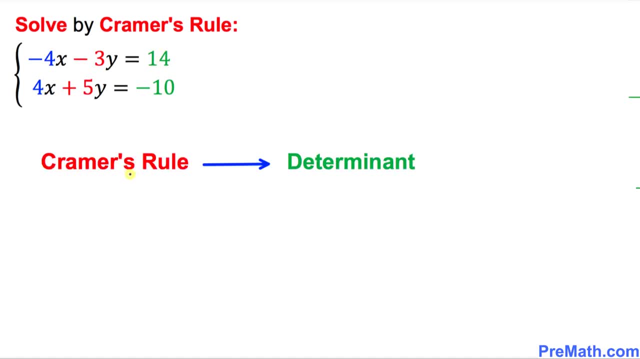 And one more thing: just keep in your mind that Kramer's rule deals with the determinants, And determinant is relative And determinant is related to matrix or matrices. Instead of brackets. this is represented by vertical bars like this way. That is pretty much it. 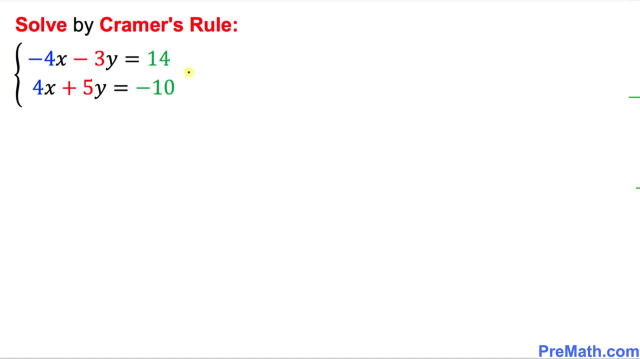 Now let's get started with the solution process, Since we want to solve this system of equations. that means we are going to find x value and we are going to find y value, And here I have nicely set these variables up: x equal to one box on the top and one box at the bottom. 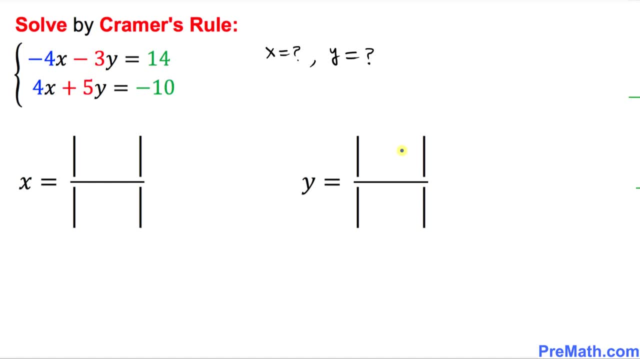 And likewise one box on the bottom and one box on the top. By the way, these boxes are called determinant, as I told you a few seconds ago. So let's start filling out these boxes. So let's get started with the left-hand side only of these equations. 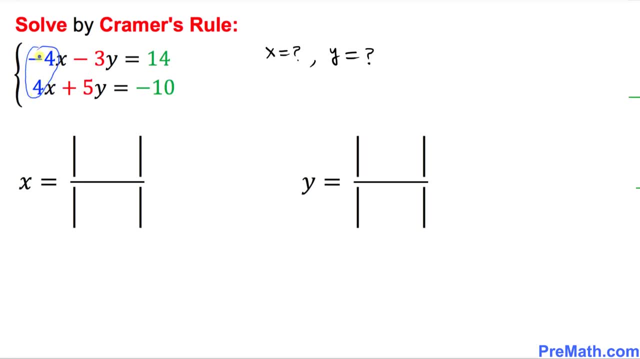 Let's focus on this, This part. the coefficient of x negative four and four is going to go at the bottom right up here, And for y coefficients, this one negative three and five is going to go right up here. 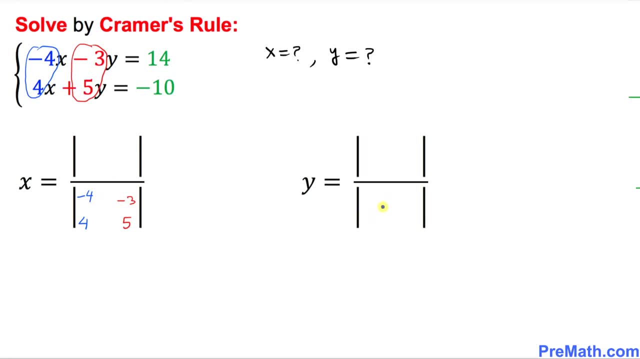 Likewise, whatever we put down, we're going to do the same thing. Bottom determinant is going to be identical: It's going to be a negative four and five, It's going to be a negative four and likewise, it's going to be negative three and five. 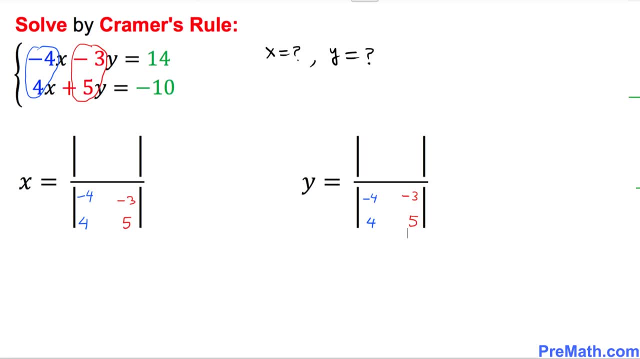 So far, so good. So now let's shift our focus on the top. You see this on the right-hand side. These are constants 14 and negative 10.. For x variable, these green numbers are going to show up on the left column. 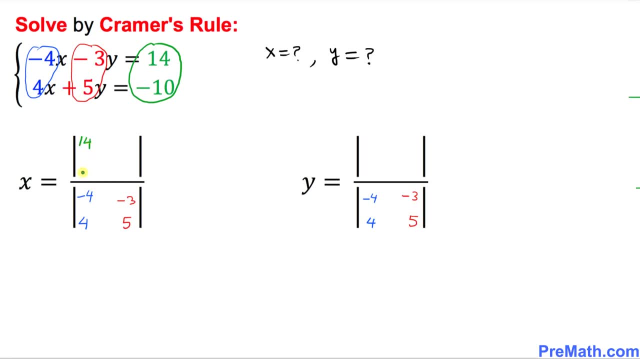 So I'm going to put down negative 14.. And for y, this is going to shift, this green number is going to shift to this next column. So 14 and negative 10.. Now we are almost done And now we are going to fill out this empty slot or empty column. 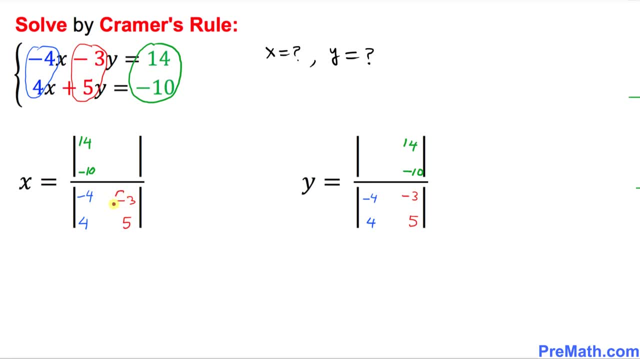 So right underneath this empty column we are going to see these red numbers. Just push them up, copy and paste them. So this is going to become negative three and five. Likewise to fill out this column over here. look at the numbers underneath it. 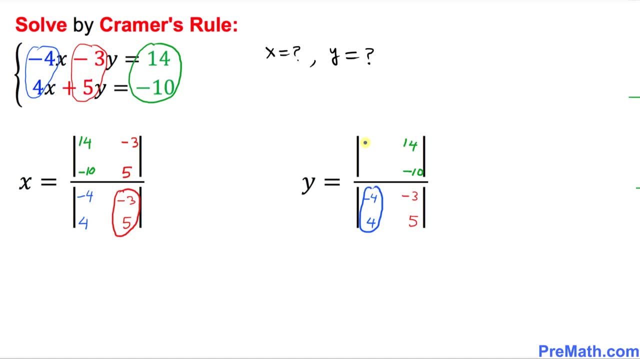 which is negative four and four. Just copy and paste them: Negative four and four. Now we are done with these filling out part. The next thing is we want to find the value of these digits. We want to find the value of these determinants. 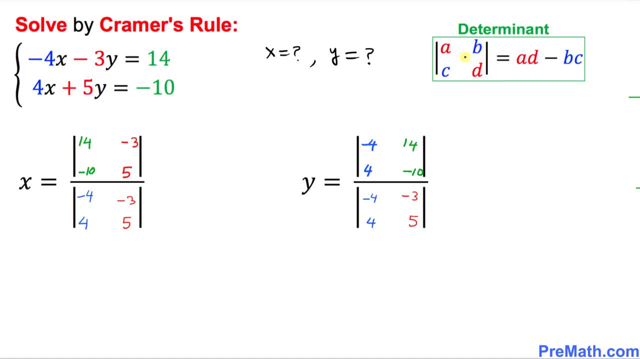 And here's the formula or the fact we're going to be using to find the value of the determinant. It says that the determinant A, B, C, D- if you want to find the value, that's going to be A times D and then minus sign and then B times C. 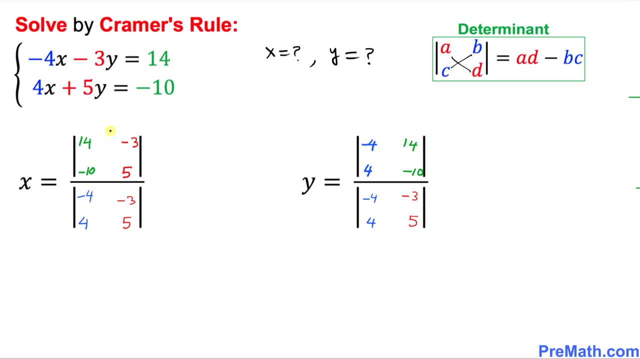 That's what I put it down. We're going to be using the same definition to evaluate these determinants. Let's get started. If we diagonally multiply this one, 14 times five equals to 70. And then we're going to put a minus sign before we do anything else. 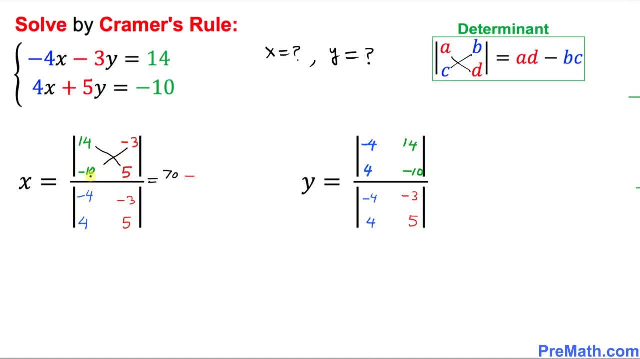 And then I'm going to cross multiply the other way around. Negative three times negative 10 equals to positive 30 divided by. we're going to do the same thing over here. Negative four times five is negative 30.. We're going to do the same thing over here. 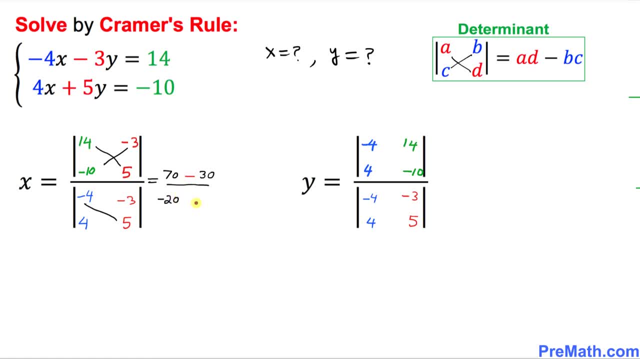 Negative 20.. And then we are going to put a minus sign before we do anything else. And then we're going to multiply the other way around: Four times negative three is negative 12.. Let's simplify this one over here. If I simplify this thing on, the top is going to be 40 divided by negative 20.. 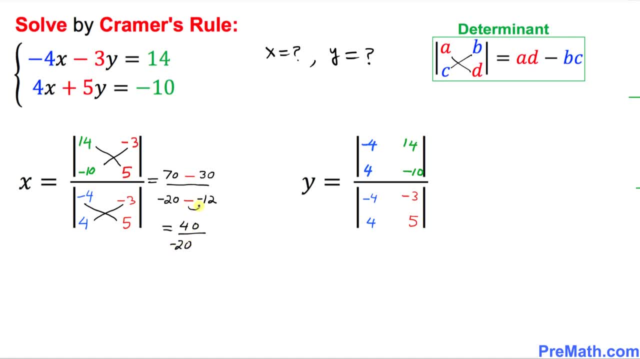 And then you see this: It's going to be negative 20. You see these two signs- negative and negative- become positive 12. So that means it's going to be 40 minus eight And if you simplify, that is going to give you negative five.